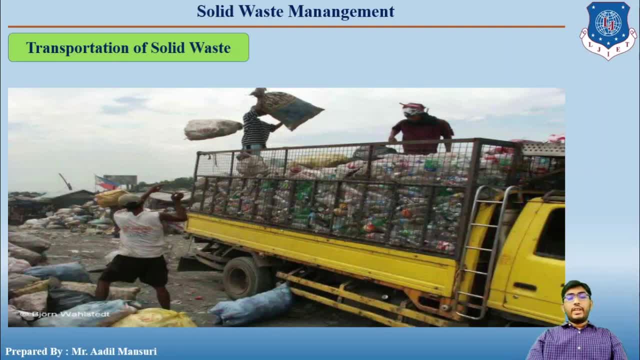 instructed by the law that the transportation must be done in closed containers. only the. the industrial waste must be transported separately and must be deposited in a safe way after suitable treatment. but it is not happening. so any type of hazardous waste should be labeled and coded so that, in case of an accident, the emergency services know how to handle the. 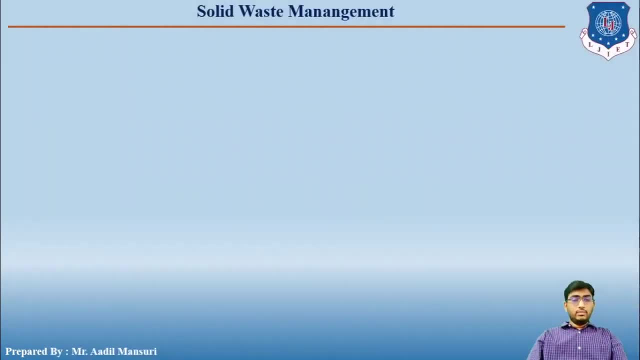 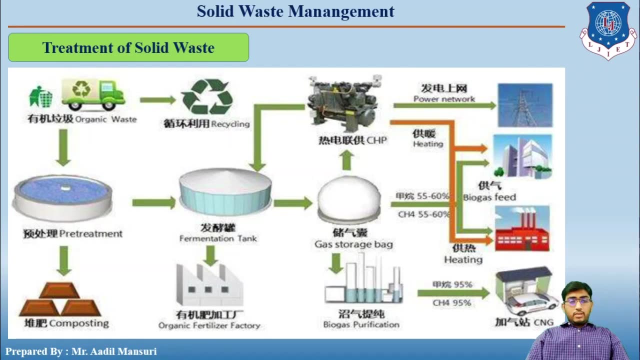 condition. okay, then, talking about treatment of solid waste. so the waste has to be treated before disposal for the protection of environment and in the treatment of biodegradable waste can be processed by composting, vermicomposting, anaerobic digestion or any other appropriate biological processes for stabilization of waste. in any case, the solid waste should be reduced. 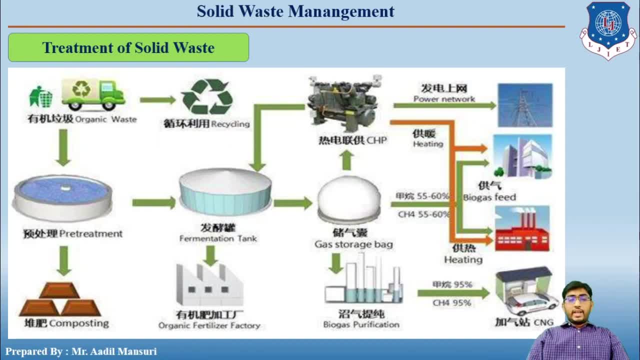 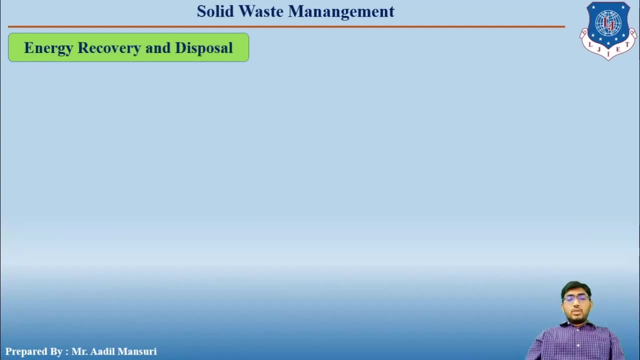 in terms of the salt and fat framing that is performed on both surfaces, but it is necessary. quantity at source segregated and then carefully transported, is transported and the economically treated before the final disposal. okay, so let us move ahead. next topic is energy recovery and disposal. so the most common method of energy recovery and disposal for non-hazardous solid 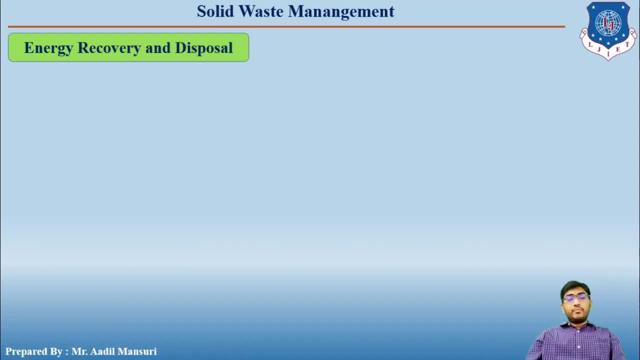 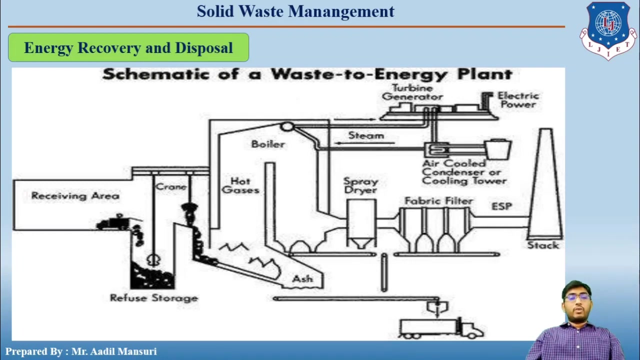 waste are incineration, composting and land filling. okay, the final disposal of waste should be done in such a way that it maintains or it remains a waste in actual sense, that is, nothing can be recovered out of it or it could not be used anywhere. okay, so this is the schematic diagram for 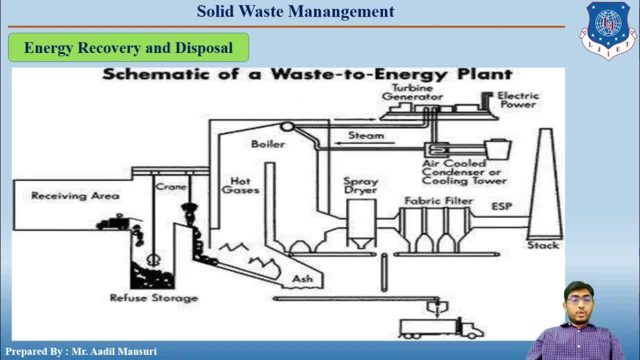 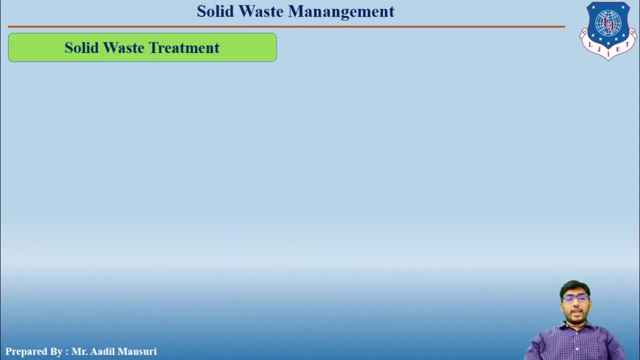 waste to energy plant. okay, so let us move ahead with the next topic, that is, solid waste. okay, so there are several treatments which are carried out in order to treat the solid waste efficiently and make it, uh, hazardless right, or make it safe for environment. so first one is the composting, then comes incineration. 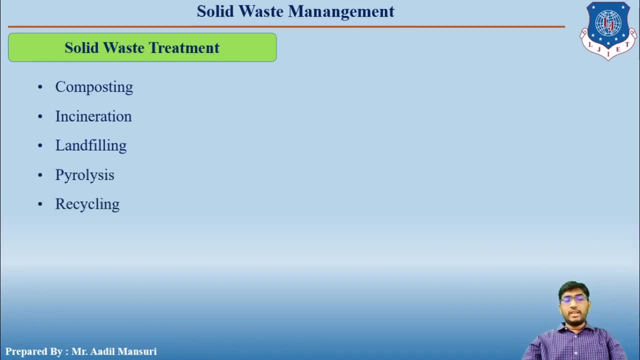 then comes land filling, pyrolysis and recycling, so we will be discussing each of them in detail. so let us start with the first one, that is, the composting. so it is a process in which organic matter of solid waste is decomposed and converted to humus. 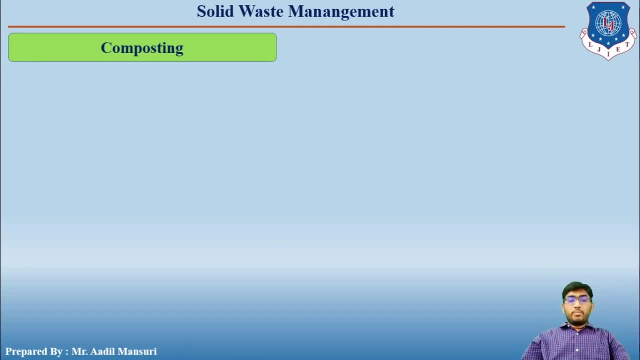 and mineral compounds. the compost at the end is used as a fertilizer. there are three different methods for composting. the first one is by trenching, second one is known as by open window composting and the third one is known as mechanical composting. let us first start with the composting by trenches, so usually three to twelve meters long. 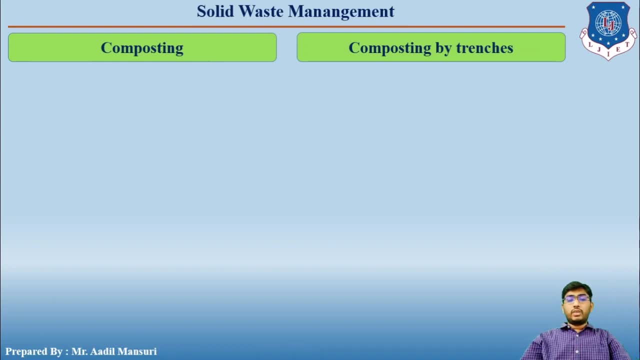 or two to three meter wide or one to two meter depth. of trench is dug with a spacing of two meters. dry wastes are filled up in 15 centimeters stack and on the top of each layer five centimeter thick sandwiching layer of animal dung is sprayed in the semi-liquid form. 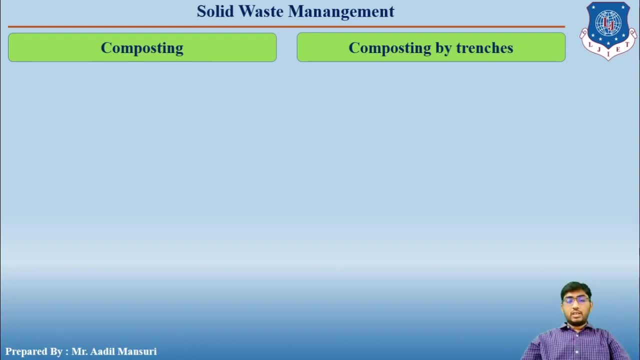 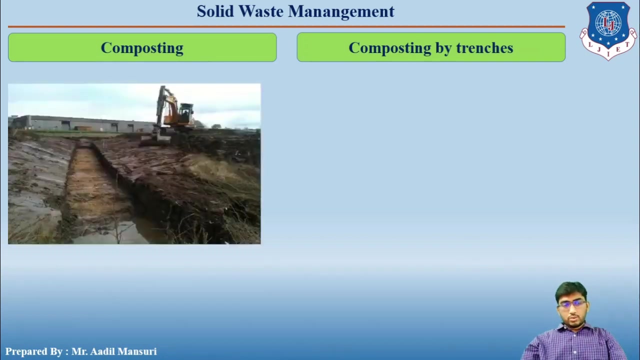 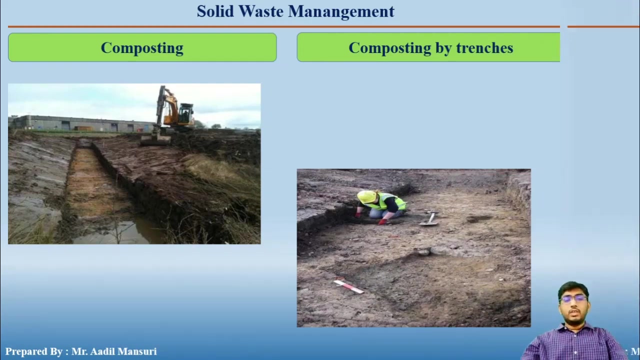 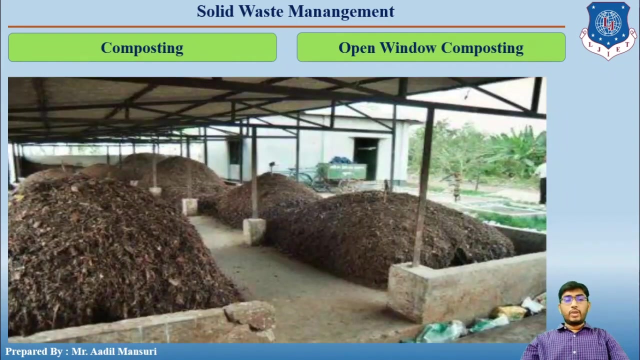 biological action starts in two to three days and decomposition then starts. this solid waste stabilize in four to six months and change into brown colored, odorless powdery form, which is known as the humus. so let me show you the pictures clear. next is open window compostig. okay, so you can see the first pictures. 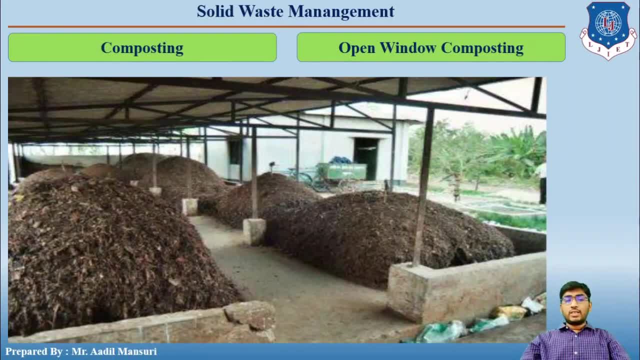 so large materials like broken glass, stone piles- uh sorry, stones- and plastic articles are first removed. remaining solid waste is dumped on the ground in the form of piles or stacks of 0.6 meters to one meter of height and the width and length of piles for some. 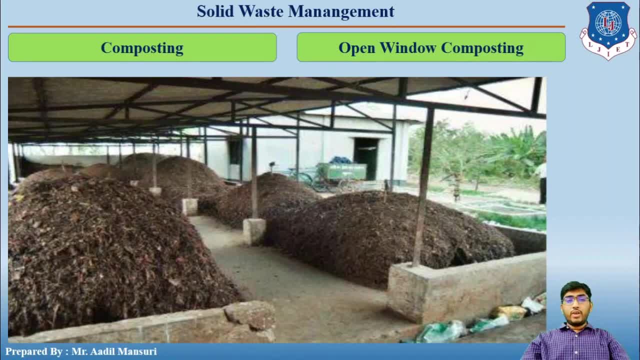 waste is gradually treating, which is observed are usually one to two meters and six meters. moisture content is maintained as sixty percent and temperature does increases inside the pile. right then it is turned for cooling and a region to avoid anaerobic decomposition, and this complete process usually takes four to six months. okay, this complete process. 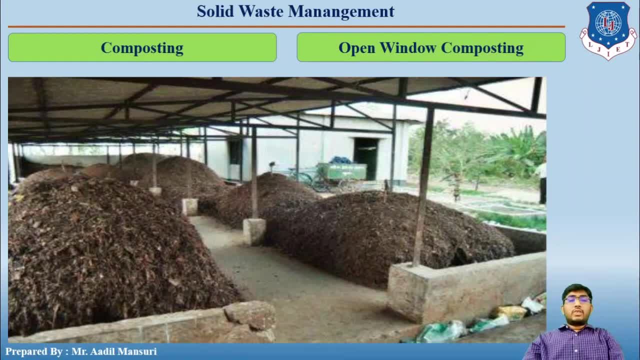 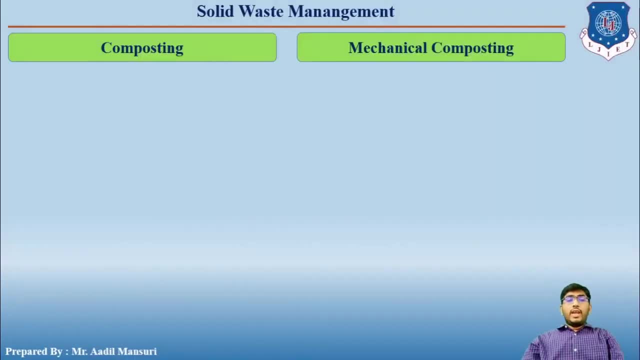 usually take four to six weeks. so let us now start with the next topic, that is, the mechanical composting. so, unlike other composting methods like trenching, open trenching or open window composting, this mechanical composting process usually takes four to six months. okay, this complete process. 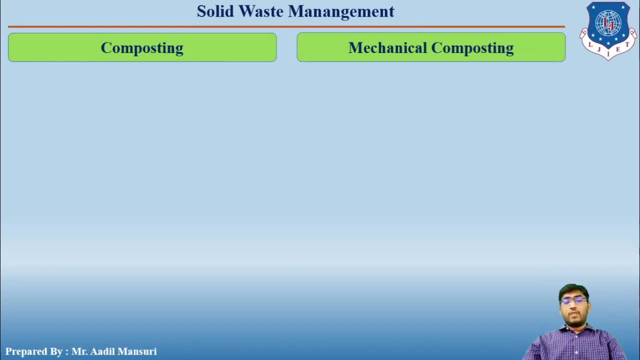 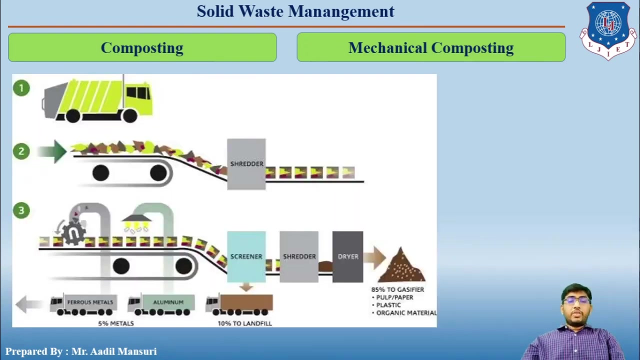 requires a less area, and the stabilization of waste takes three to six days. so the operations usually involved are reception of the refuse, segregation, shredding, stabilization and making of the humans. okay, so you can see the picture. okay, students. so let us now move towards the next topic. so let's. 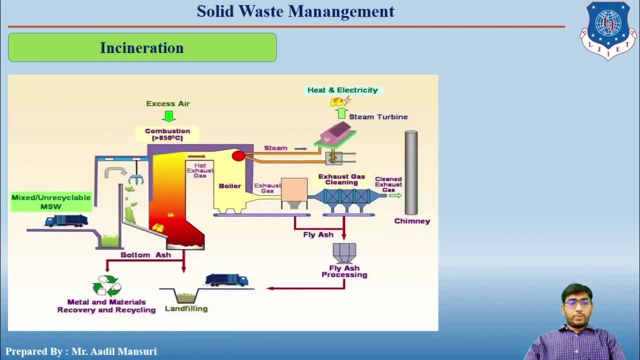 start with the incineration. so let me first show you the picture of incineration. okay, so Incineration is a waste treatment process that involves the combustion of organic substances contained in waste material. incineration and other high-temperature waste treatment systems are described as thermal. 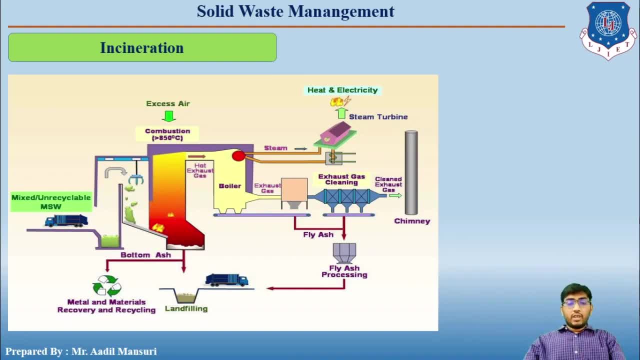 treatments and incineration of waste material converts waste into ash, flue gases and heat. okay, so incinerations are used for this process. only now important points get to know regarding the dad wrap process and through this process of consideration are used only now. important points, just If you do, theόσpecial mention was the and heat. fine, so insulations are used on this process. 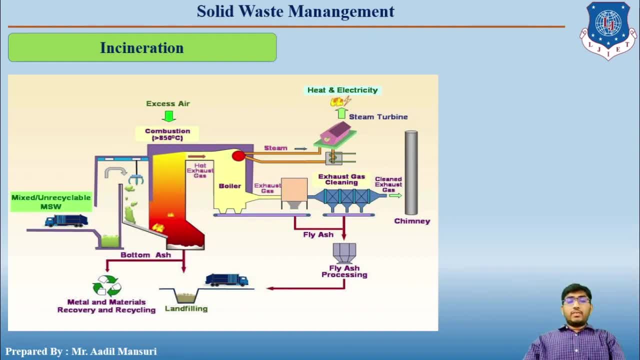 okay, so incinerations are used on this process only now. important points: you should do know that there may be process only now. important points regarding incineration are: supplying of the solid waste should be continuous. waste should be proper mixed with fuel for complete combustion and 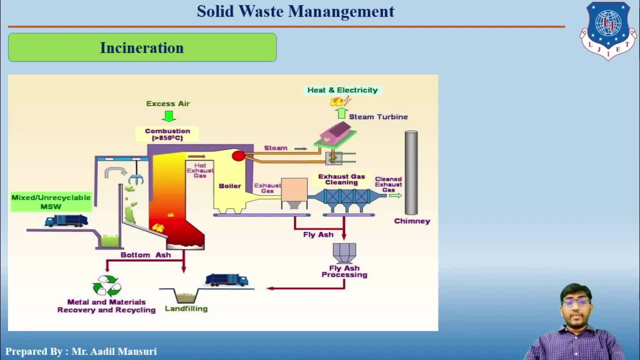 temperature should not be less than 670 degree centigrade. next, talking about its advantages, its most hygienic method: complete destruction of the pathogens takes place, no odor nuisance, heat generated may be used for steam power plant and clinkers used or produced may be. 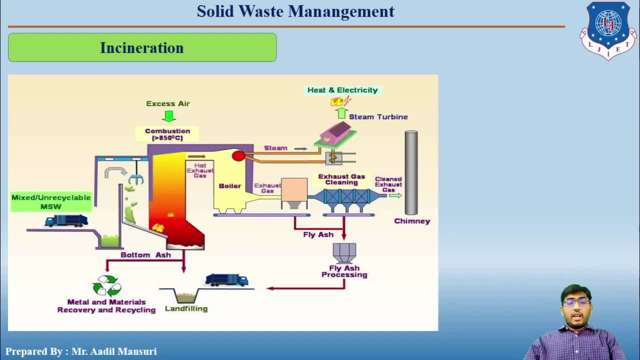 used for road constructions. less space is required and adverse weather conditions also has no effect on the incineration. okay then, talking about the disadvantages- large initial expenses- are there care and attention required? otherwise incomplete combustion bill, which should be setup for proper use, can also be considered as a subject of discussion. 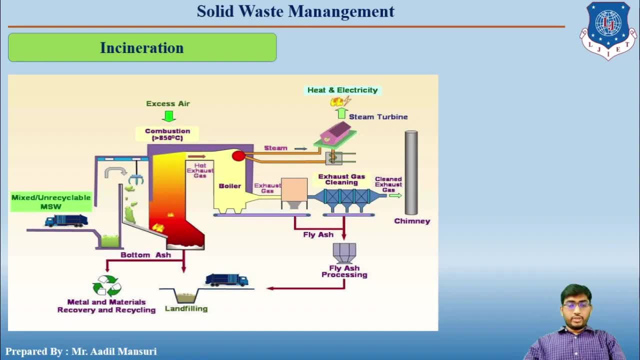 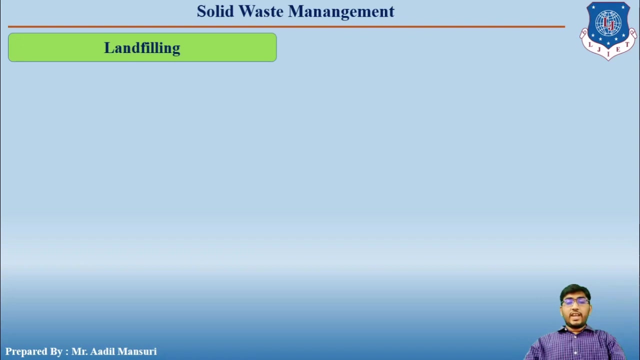 take place right, which will increase the air pollution and residues required to dispose, which required more money and, lastly, large number of vehicles required for transportation. okay, so next is landfilling. so a landfill site is a site for the disposal of waste materials by burial and is the oldest form of waste. 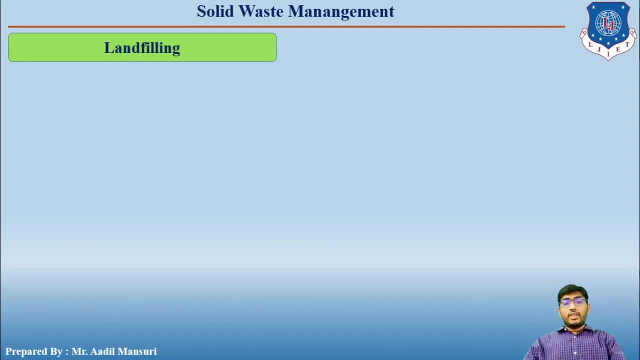 treatment. historically, landfills have been the most common methods for organized waste disposal, and remain so in many places around the world right now. the dumping is done with the layers of one to two meters, and the layer is covered with the soil of 20 centimeter thickness. this is the picture for modern. 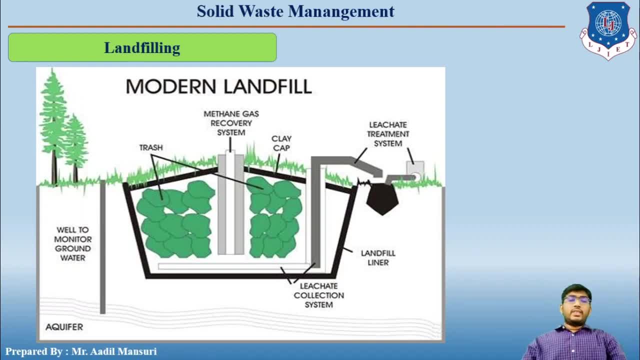 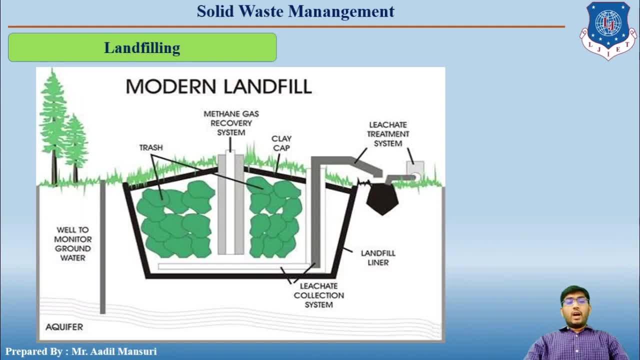 disposed of. no separation is required, unused land can also be used, and methane gas which is produced with this process can be used as a fuel. right, it does have several disadvantages, which include that it requires a large land- okay, large area of land is required, then. proper management of the land is required, then proper. 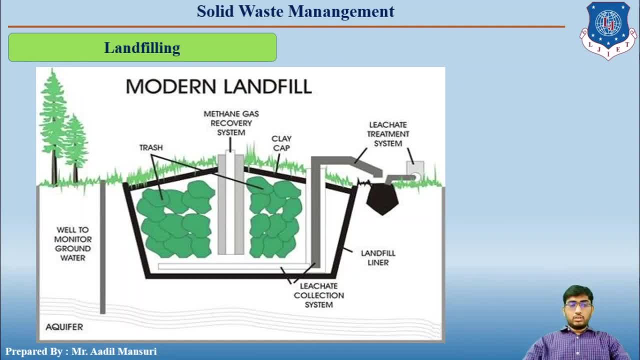 of land is required, then proper management of the land is required, then proper dumping site may not be available because there is chances that there are dumping site may not be available because there is chances that there are chances that in the vicinity certain or in the nearby residential area is there. 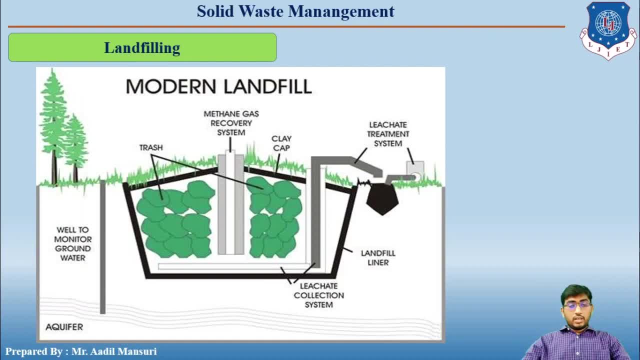 chances that in the vicinity, certain or in the nearby residential area is there. right then there is an order nuisance right and use of insecticide is required. right then there is an order nuisance right and use of insecticide is required or otherwise, there will be more insects and flies which will be generated. 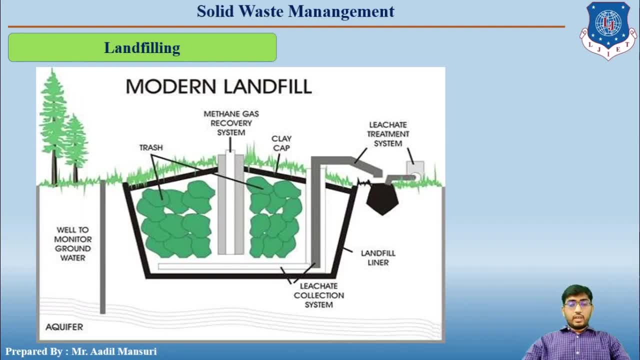 or otherwise, there will be more insects and flies which will be generated. leachate should be collected regularly. right leachate: I have explained it's. a leachate should be collected regularly. right leachate: I have explained it's a colored leachate should be collected regularly. right leachate: I have explained it's a. 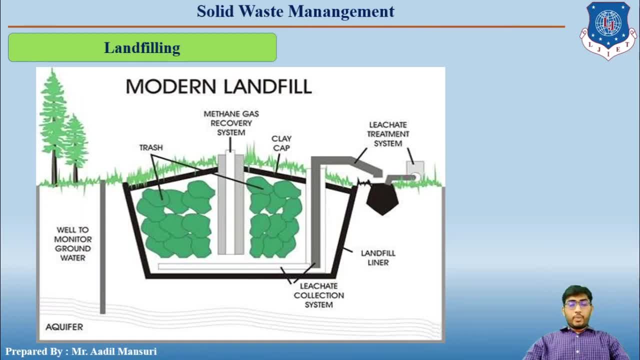 colored leachate should be collected regularly. right leachate: I have explained. it's a liquid, then methane gas should be collected properly. and greenhouse gases liquid, then methane gas should be collected properly and greenhouse gases liquid, then methane gas should be collected properly and greenhouse gases problem also arises. okay, so next is: 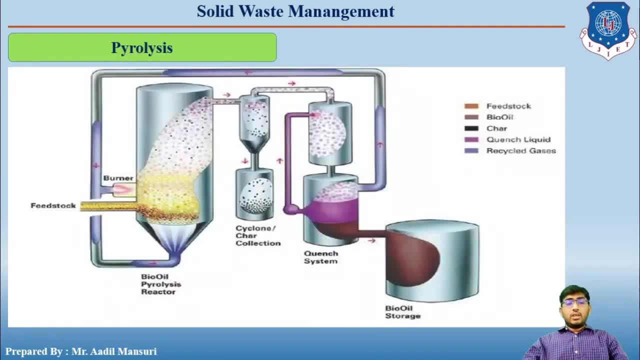 problem also arises, okay. so next is: problem also arises, okay. so next is pyrolysis, so it is the heating of solid pyrolysis. so it is the heating of solid pyrolysis, so it is the heating of solid waste at a very high temperature in. 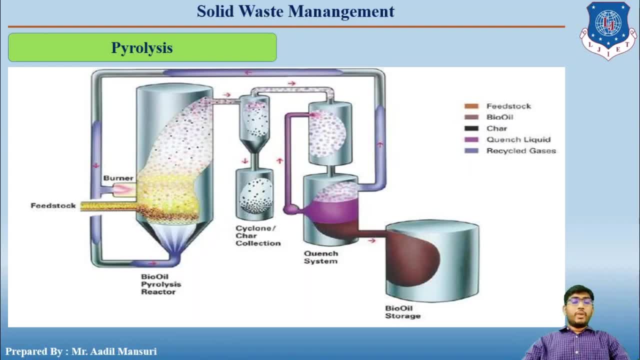 waste at a very high temperature, in waste at a very high temperature, in absence of air, which is usually carried. absence of air, which is usually carried. absence of air, which is usually carried out between 500 degree centigrade to 1000 out between 500 degree centigrade to 1000. 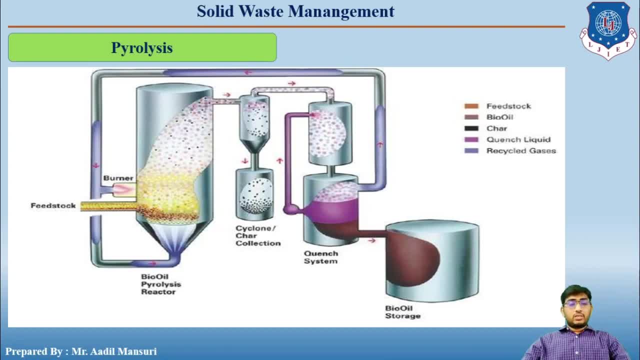 out between 500 degree centigrade to 1000 degrees centigrade gas liquid and degrees centigrade gas liquid and degrees centigrade gas liquid. and chaos are the main by-products. fine, okay, chaos are the main by-products. fine, okay, chaos are the main by-products. fine, okay, students. so let us now start with the 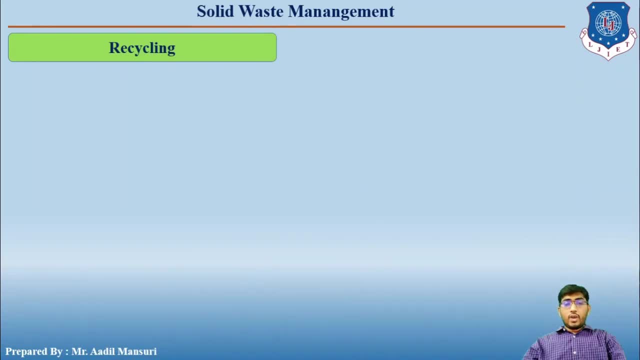 students. so let us now start with the students. so let us now start with the next one, that is the recycling. okay. next one, that is the recycling. okay. next one, that is the recycling. okay. recycling is a process to produce new. recycling is a process to produce new. 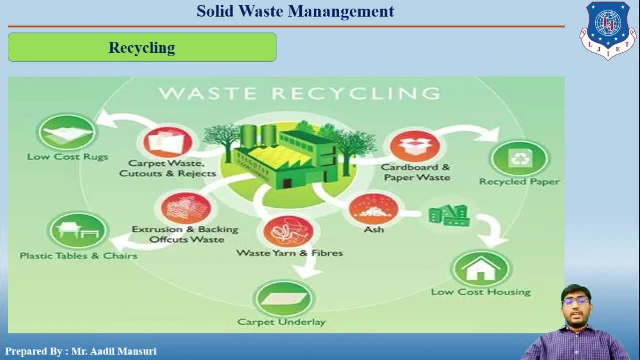 recycling is a process to produce new products from the used material right. it products from the used material right. it products from the used material right. it reduces the consumption of fresh raw. reduces the consumption of fresh raw, reduces the consumption of fresh raw materials and reduces energy usage. 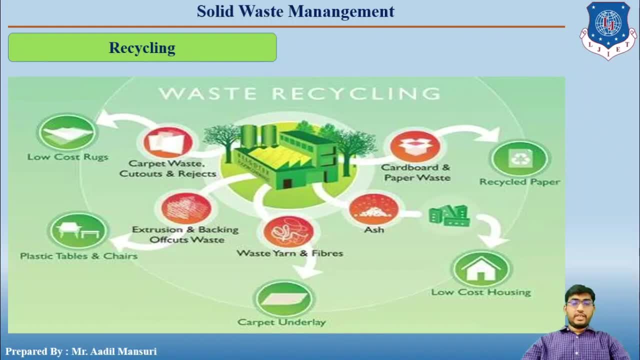 materials and reduces energy usage. materials and reduces energy usage. reduces air pollution right from. reduces air pollution right from. reduces air pollution right from incineration and water pollution. water incineration and water pollution. water incineration and water pollution. water pollution from land filling right now. 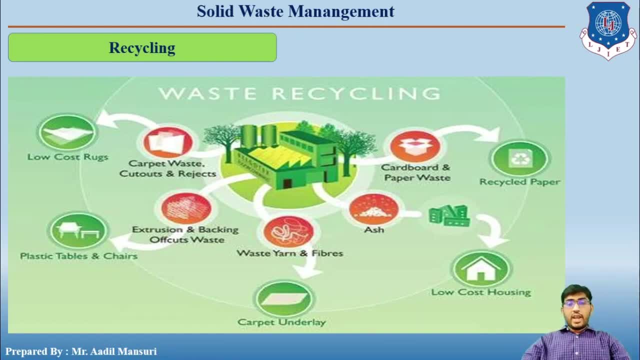 pollution from land filling right now. pollution from land filling right now. recycling is a key component of modern recycling, is a key component of modern recycling, is a key component of modern waste reduction and is the third waste reduction and is the third waste reduction and is the third component of the reduce, reuse and recycle. 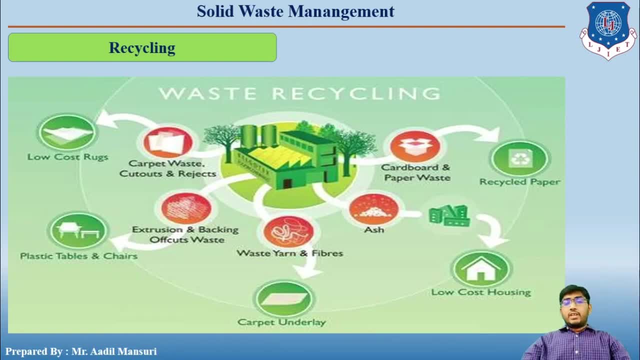 component of the reduce, reuse and recycle. component of the reduce, reuse and recycle waste hierarchy. okay, recyclable waste hierarchy. okay, recyclable waste hierarchy- okay. recyclable materials include many kinds of glass materials. include many kinds of glass materials. include many kinds of glass papers, but metals, plastic, textiles and 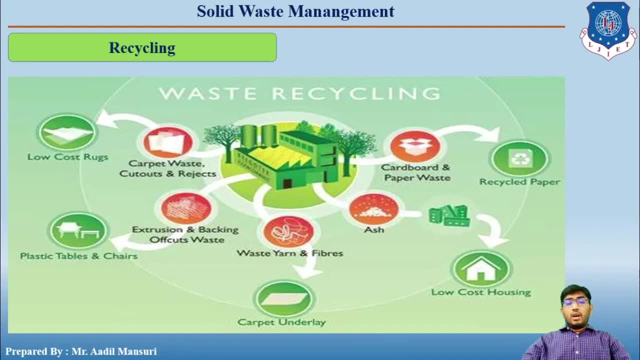 papers but metals, plastic, textiles and papers but metals, plastic, textiles and electronics. okay then, although similar in electronics. okay then, although similar in electronics. okay then, although similar in effect. the composting or other reuse effect. the composting or other reuse effect, the composting or other reuse of biodegradable waste, such as food or 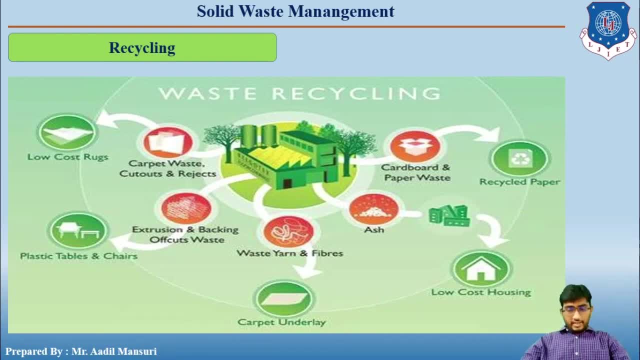 of biodegradable waste such as food, or of biodegradable waste such as food or garden waste is not typically considered. garden waste is not typically considered. garden waste is not typically considered for recycling: okay, and materials to be for recycling: okay, and materials to be for recycling: okay and materials to be recycled are either brought to a: 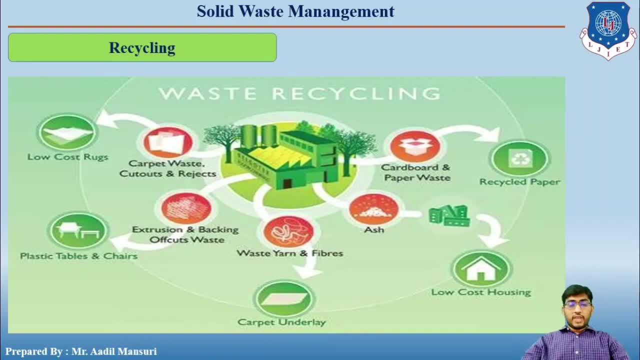 recycled are either brought to a recycled are either brought to a collection center or picked up from the collection center. or picked up from the collection center or picked up from the curbside, then sorted clean and processed curbside, then sorted clean and processed curbside, then sorted clean and processed into new materials. okay, so, my dear, 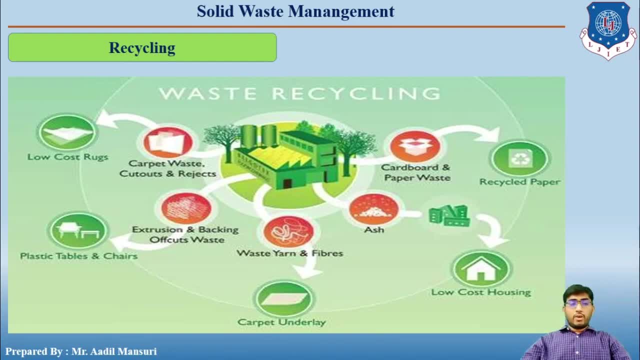 into new materials. okay so, my dear, into new materials. okay. so, my dear students, this is the end of this, students, this is the end of this, students, this is the end of this particular module that is solid waste, particular module. that is solid waste particular module, that is solid waste management. and we will start with the